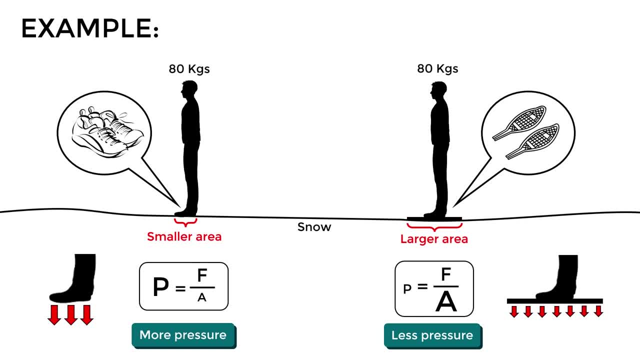 will exert less pressure on the snow. For this reason, the person on the left will tend to sink into the snow, while the person on the right will be able to walk more easily. So now that we have seen the general concept of pressure, let's move on to. 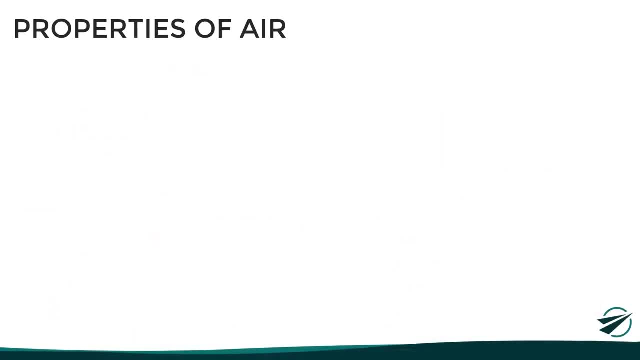 atmospheric pressure. But first let's remember the main properties of air. As we said in a previous video, air is a fluid composed of various gases and its main properties are temperature, pressure, density and humidity. And although in this video we will focus on the 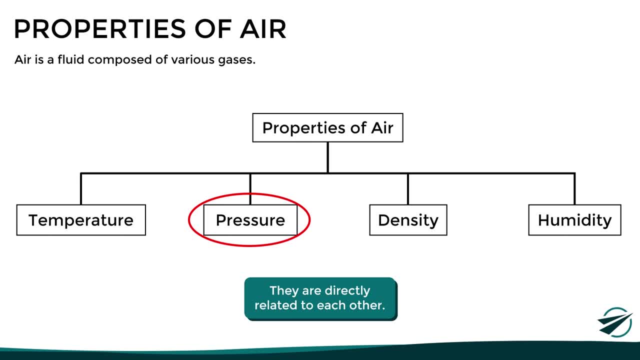 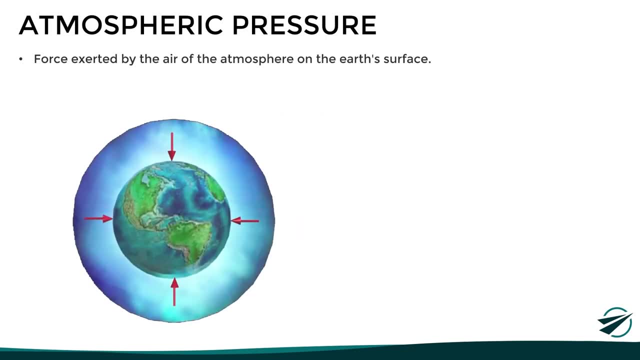 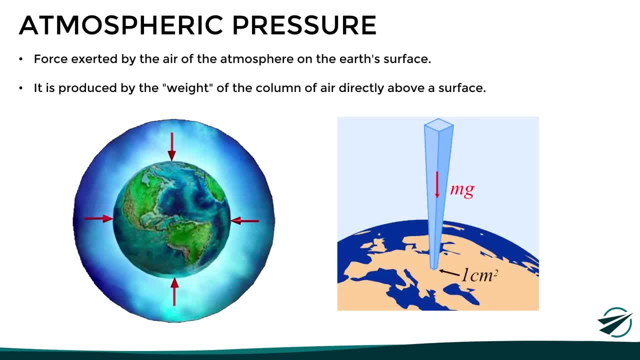 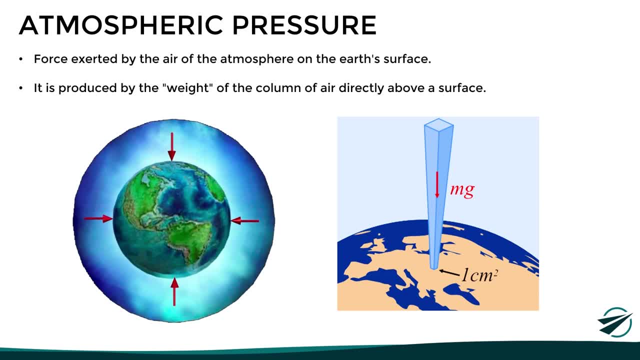 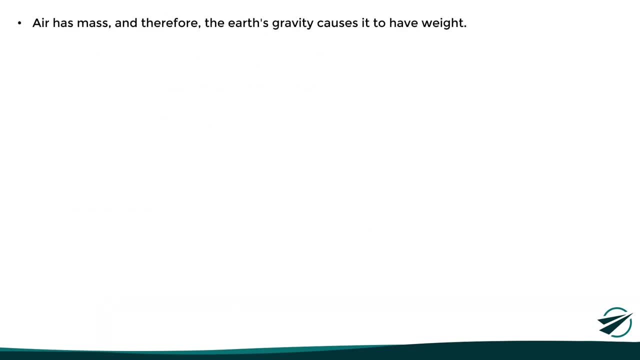 Now this concept may sound rather abstract, since in practice and in our daily life, it seems that air has no weight. However, the truth is that the air has mass and therefore the earth's gravity causes it to have weight. This means that each air molecule exerts a certain 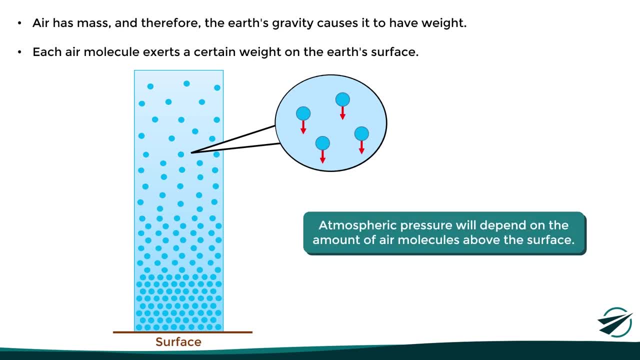 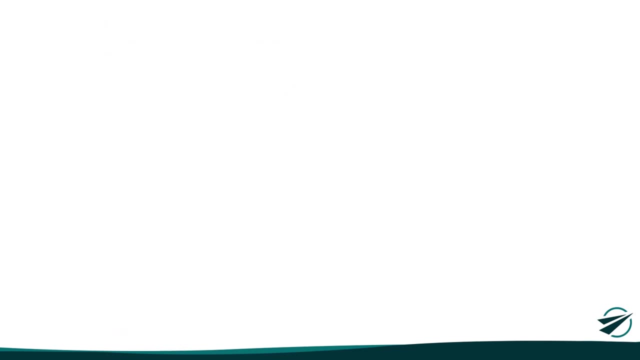 weight on the earth's surface and therefore we can affirm that atmospheric pressure will depend on the amount of air molecules above a surface. Now you might be wondering: if air has weight, why don't we feel it pushing us down against the surface? Well, the thing is that, as with all, 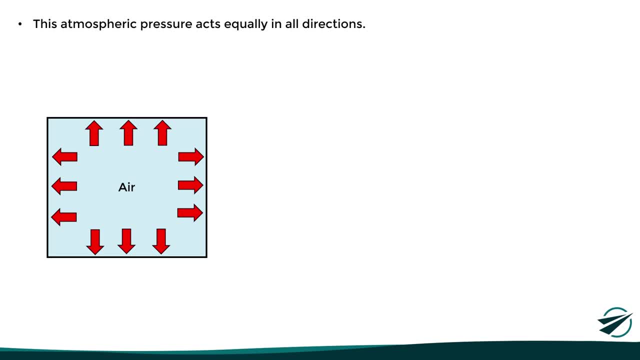 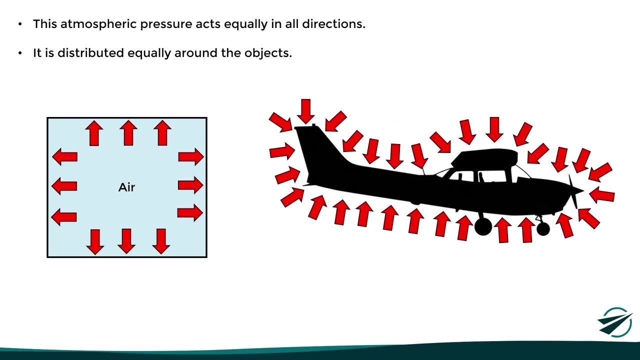 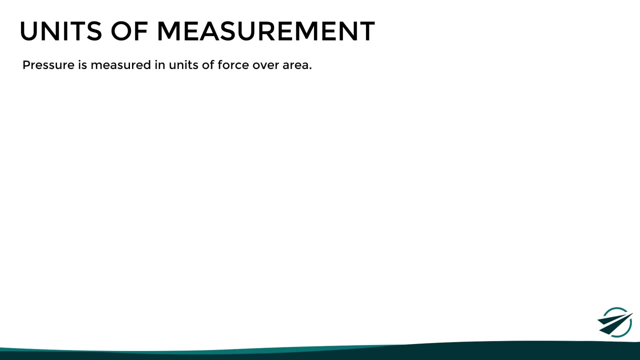 fluids. this atmospheric pressure acts equally in all directions. This means that it is distributed equally around all the objects inside the atmosphere, and this is the reason why we don't feel the atmospheric pressure. So, having understood the concept of atmospheric pressure, let's look at the units of measurement used for it. As we said previously, pressure is equal to. 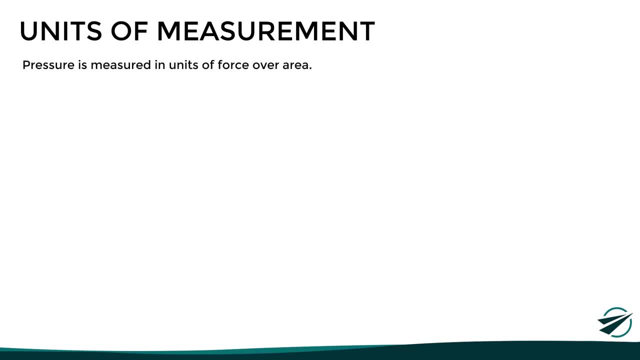 force over area. Consequently, the units of measurement to be used must take this relationship into account. The international system of units uses the Pascal as a standard, which is equal to 1 newton per square meter, As we can see, a unit of force over a unit of area. However, in meteorology, 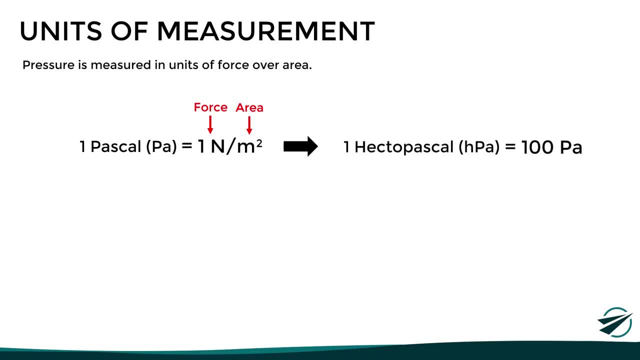 to measure atmospheric pressure, the hectopascal is often used, which is equal to 100 pascals. However, the hectopascal is not the only unit of measurement used. Other widely used units are: pounds per square inch, millibers. inches of mercury. 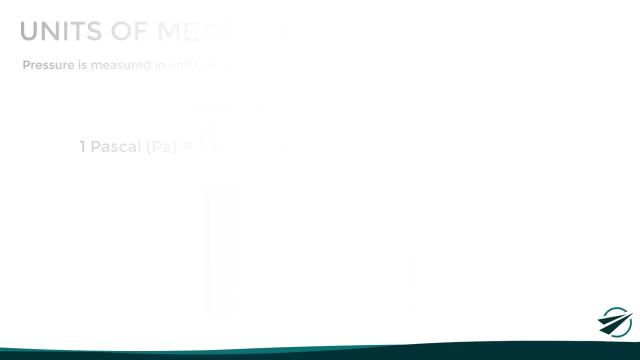 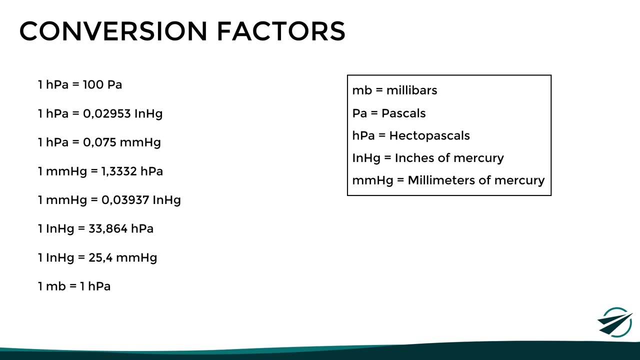 and millimeters of mercury. Here is a list of the most commonly used conversion factors between these units. Now it is important to mention that in aeronautical meteorology the most commonly used units are hectopascals and inches of mercury. And a general rule of thumb. 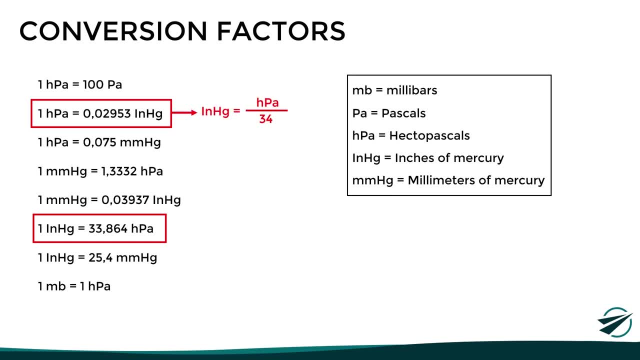 for quick conversions between these units is to divide by 34 to go from hectopascals to inches of mercury, or multiplied by 34 to go from inches of mercury to hectopascals. Now, another thing to keep in mind is that in some cases you will see the terms hectopascals and millibars used. 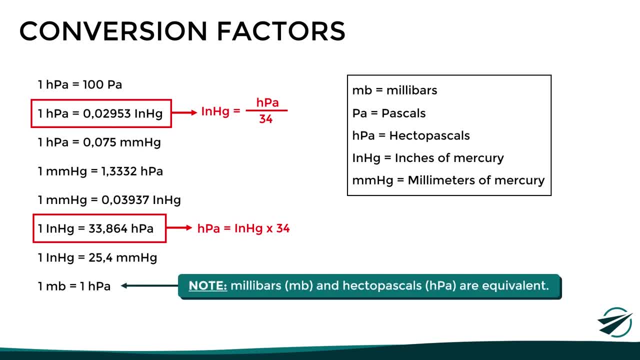 interchangeably, And this is because these units of measurement are equivalent, so there is no difference between using one or the other. So, having said that, let's look at the units of measurement used. Having seen all this, let's move on to the instrument used to measure atmospheric pressure. 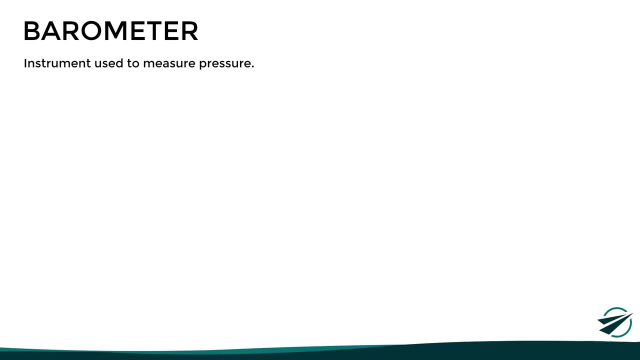 which is the barometer. However, there are different types of barometers. In fact, we can classify them into two main types: the aneroid and the mercury barometer. This last one is further subdivided into the fixed cistern, or Q barometer, and the adjustable cistern, or 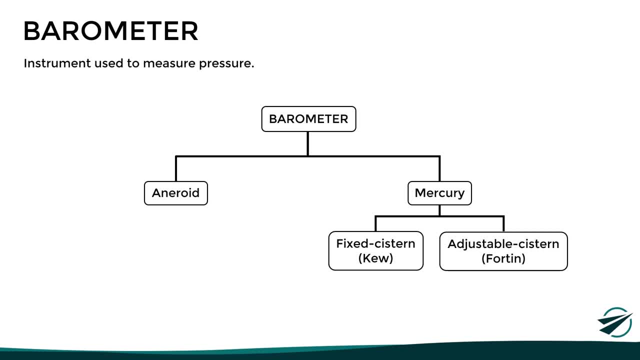 Fortin barometer. Now, although we will not go into detail on the differences between these two variants of the instrument, we will be able to see the difference between the two variants of the instrument. Let us look at the basic principle of operation of the mercury barometer. 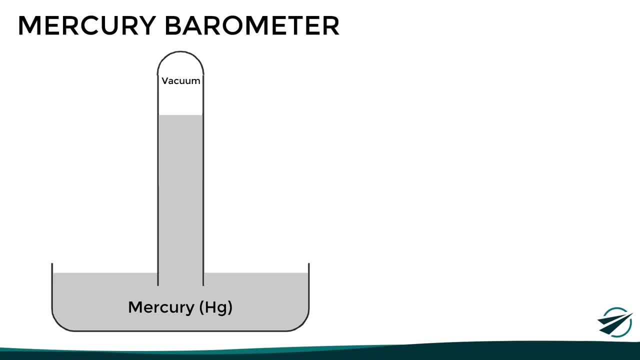 A mercury barometer consists of a vacuum glass tube that is closed at the top and open at the bottom And, as we can see, the tube is partially submerged in a bucket or cistern filled with mercury. This way, atmospheric pressure will push the mercury in the cistern, forcing it up the tube. 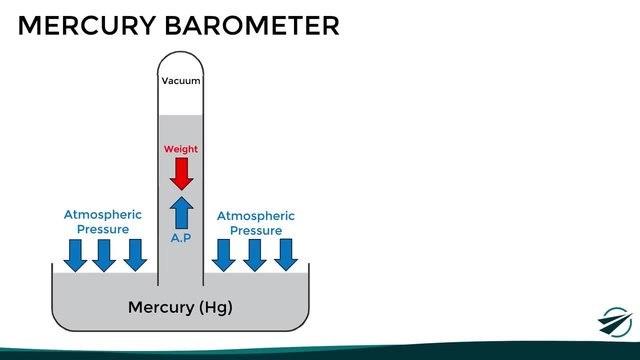 but at the same time the weight of the mercury itself will try to counteract this. The height of the mercury column depends directly on the atmospheric pressure. For example, if atmospheric pressure reduces, then the height of the mercury column in the tube will. 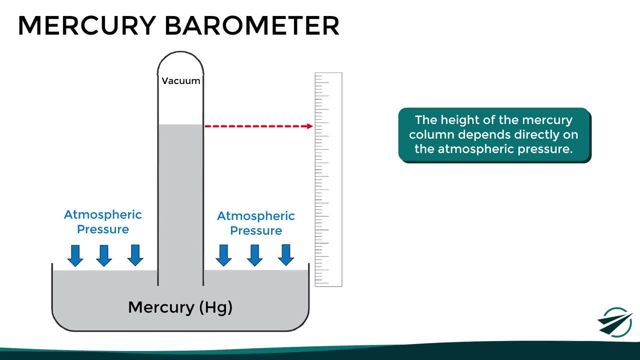 decrease, While on the other hand, if the pressure increases, the height of the mercury column will increase. Taking all this into account, atmospheric pressure can be determined directly by measuring the height of the mercury column in the tube, either in millimeters or in inches, And actually 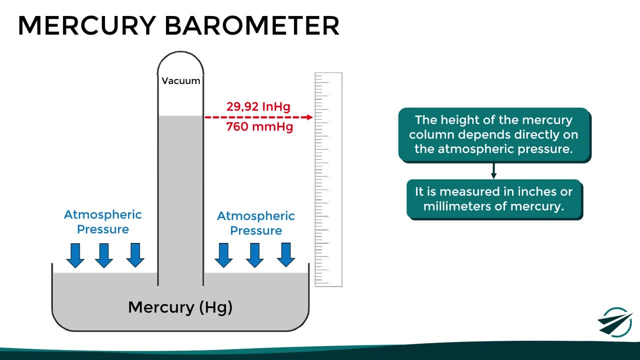 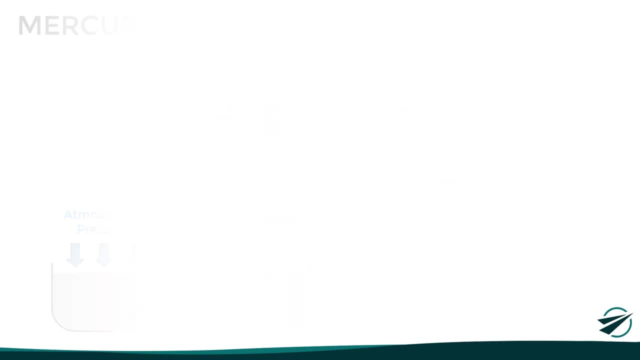 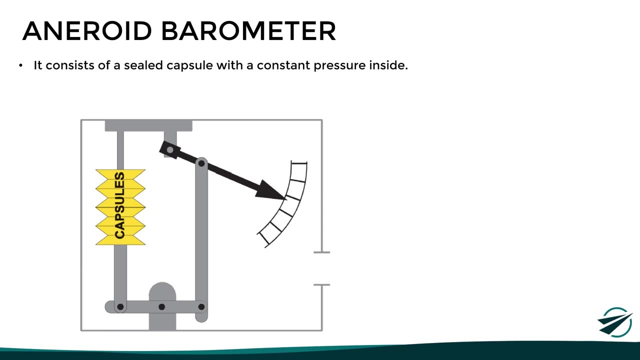 this is how the units of measurement of inches of mercury and millimeters of mercury were born. So now that we have seen how a mercury barometer works, let's move on to the aneroid barometer. This instrument consists of a sealed capsule with a constant pressure inside, And it is designed so. 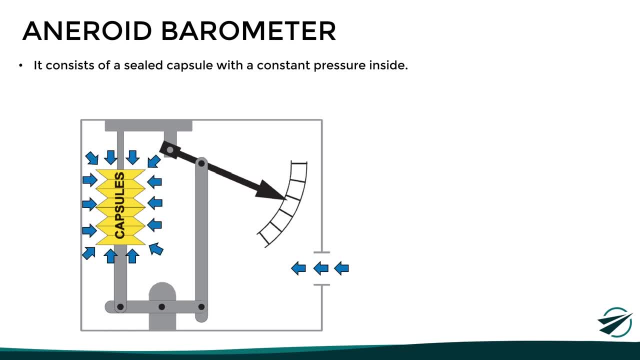 that atmospheric pressure can enter the instrument and try to compress the capsule. This way, the capsule will expand and contract depending on atmospheric pressure changes. And since this capsule is connected by means of gears to the needle on the dial, the corresponding value of the 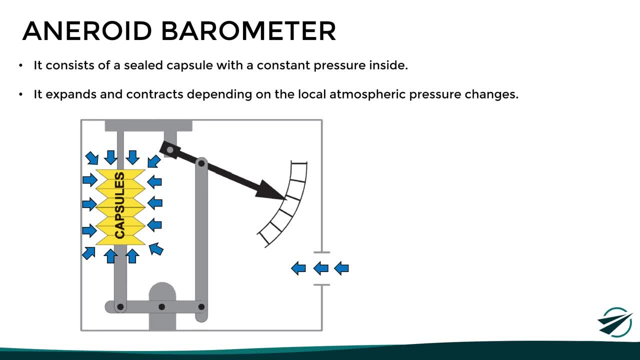 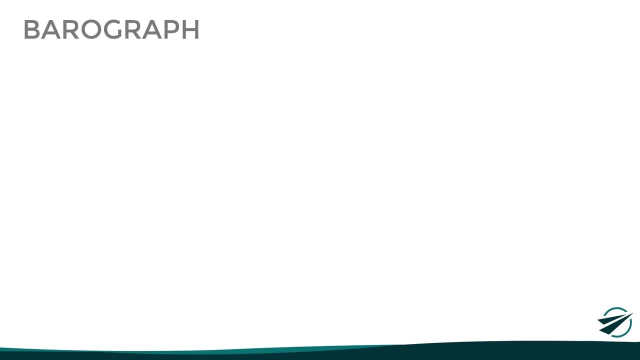 atmospheric pressure will be indicated. And, as an important fact, this exact same principle is the one used by barometric altimeters, But instead of indicating the pressure, they are calibrated to indicate the corresponding altitude. So, with this being said, let's look at the barograph. 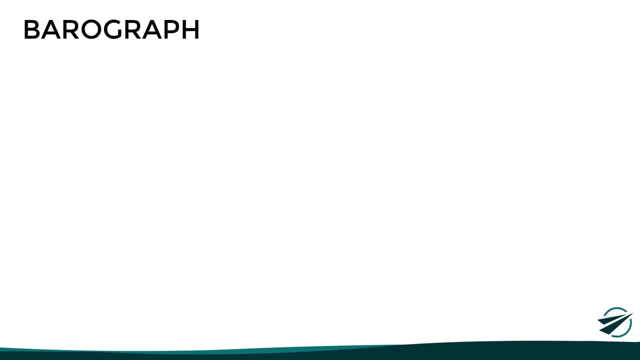 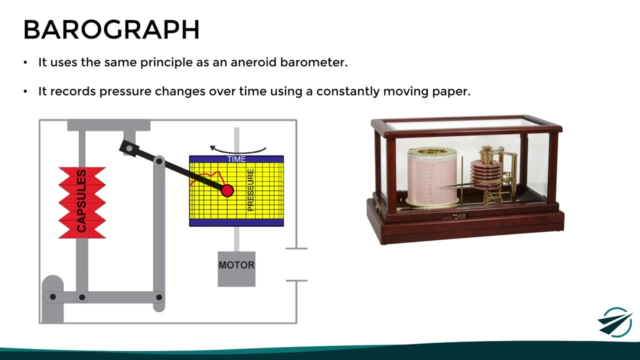 which is an instrument used to record pressure changes over time. In simple terms, it uses the same principle as the barometer. The barometer is an instrument used to record pressure changes over time. In simple terms, it uses the same principle as an aneroid barometer, But the difference is that it not only indicates, but also records. 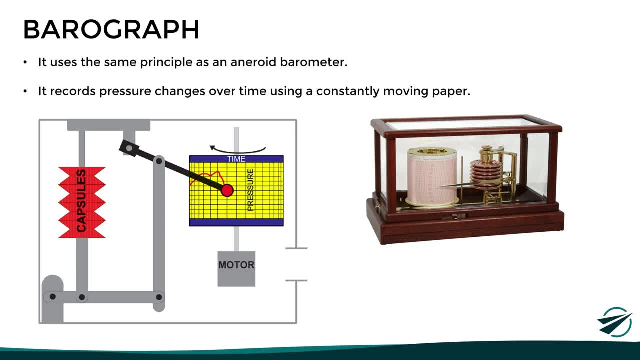 pressure changes over time. using a constantly moving paper, This instrument is very useful for identifying certain behaviors or pressure change trends within a certain period of time and therefore allow for more accurate weather forecasts and models. We must emphasize that atmospheric pressure plays a major role in the development of atmospheric conditions, and it is 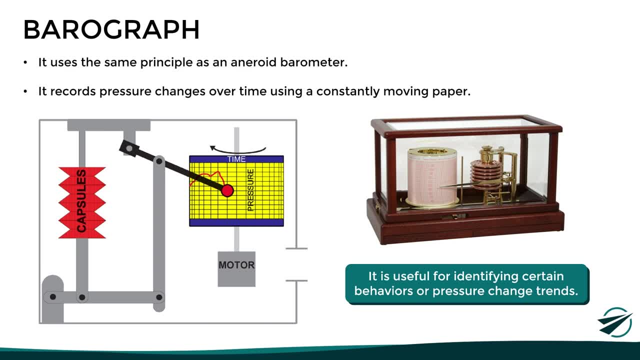 therefore important to know how atmospheric pressure affects atmospheric conditions, And it is therefore important to know how atmospheric pressure affects atmospheric conditions. and it is therefore important to know how atmospheric pressure affects atmospheric conditions, and it is therefore important to know how to read and interpret changes in pressured using the barometer and the barograph. 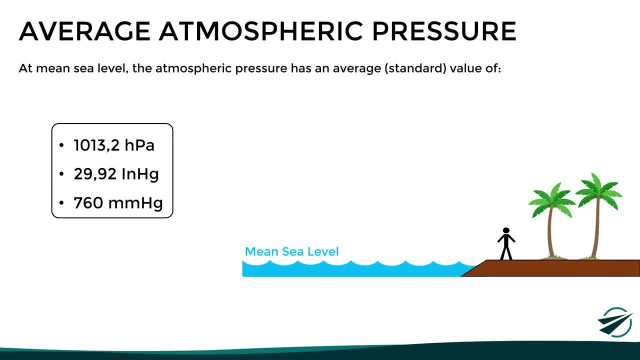 Now, in general, we can say that at sea level, atmospheric pressure has an average standard value of 1013 hectopascals, 29.92 inches of mercury or 760 mm of mercury. However, we must keep in mind that the pressure is constantly changing and therefore these are reference values only.